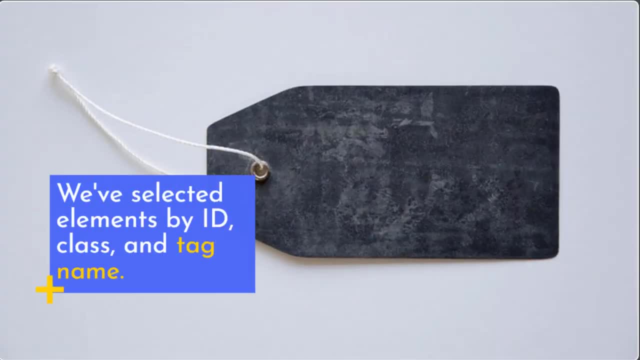 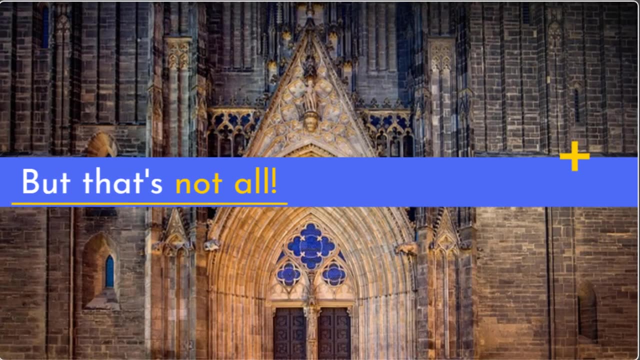 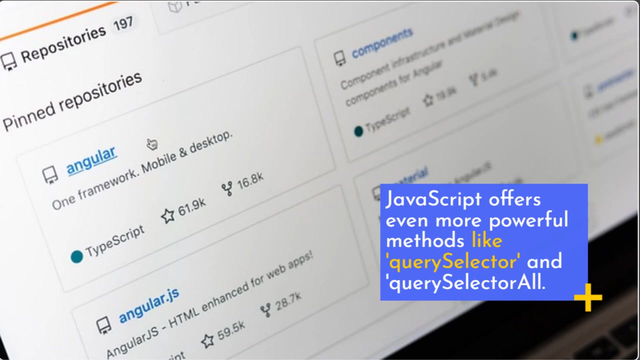 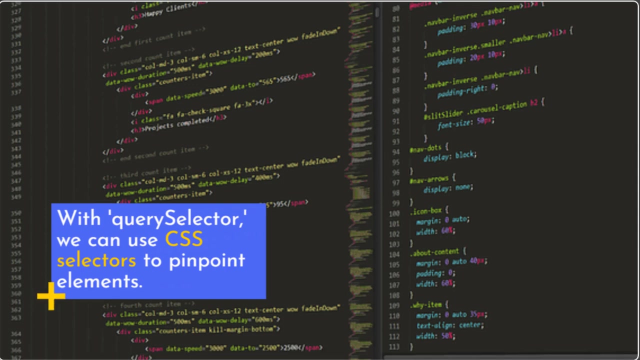 Voila. We've selected elements by ID, class and tag name, But that's not all JavaScript. JavaScript offers even more powerful methods like QuerySelector and QuerySelectorAll. With QuerySelector, we can use CSS selectors to pinpoint elements. 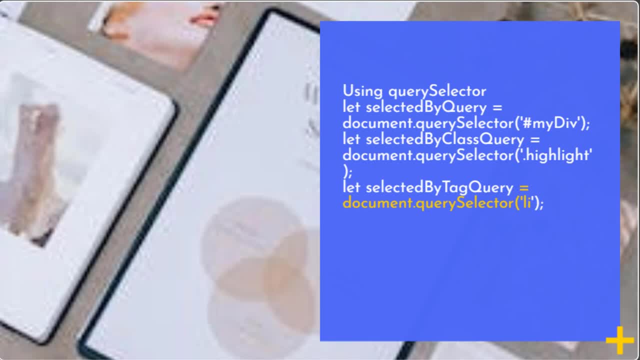 Using QuerySelector: Let's select it by query: equals document: querySelector- hashtag my div. Let's select it by class: query equals document- querySelector- highlight. Let's select it by tag: query equals document- QuerySelector- leave. Let's select it by tag: query equals document: querySelector- hashtag my div. 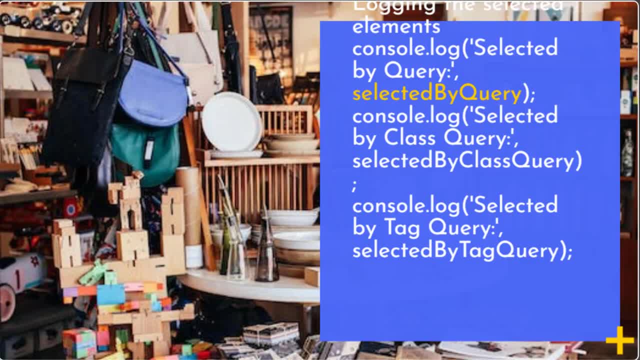 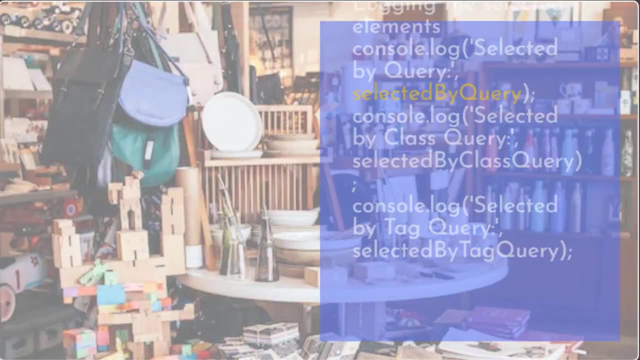 Logging the selected elements: Consolelog, selected by query. selected by query. Consolelog selected by class query. selected by class query. Consolelog selected by tag query. selected by tag query. See how concise and flexible it is: QuerySelector. 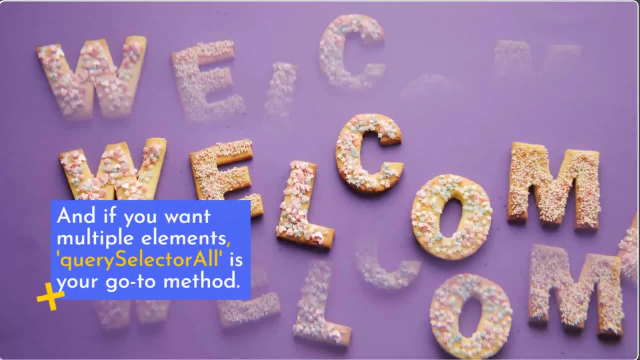 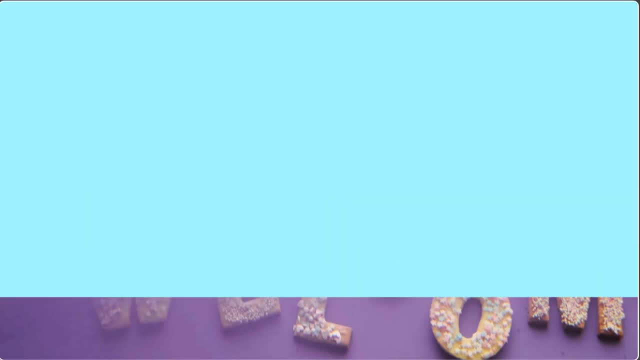 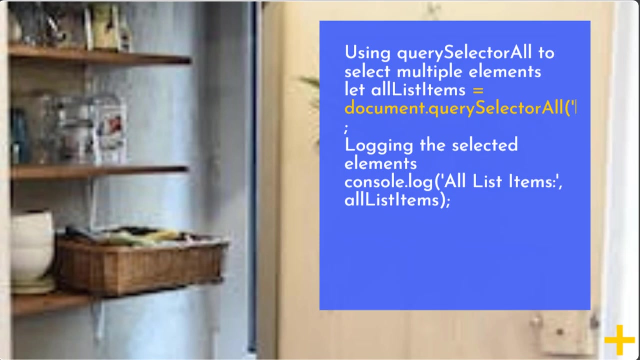 QuerySelector is a game changer And if you want multiple elements, QuerySelectorAll is your go-to method. Let's use QuerySelectorAll to select all list items. Using QuerySelectorAll to select multiple elements, Let allListItems equals document QuerySelectorAllly. 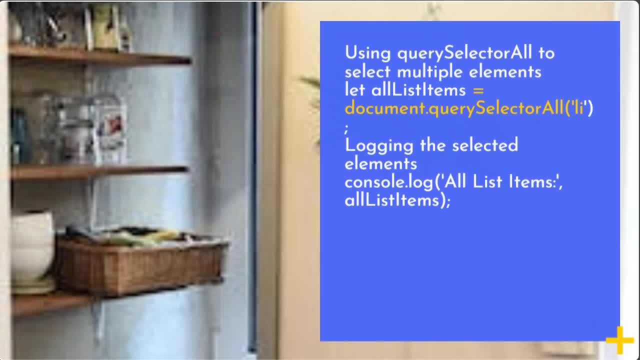 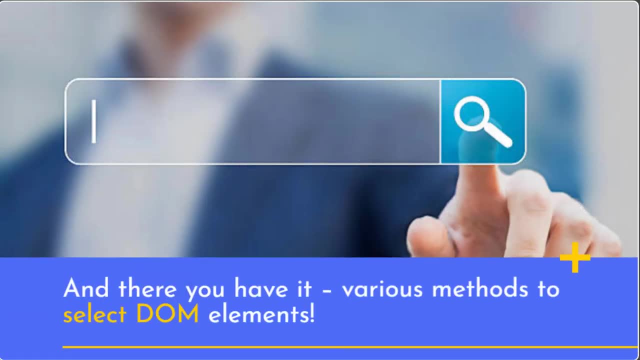 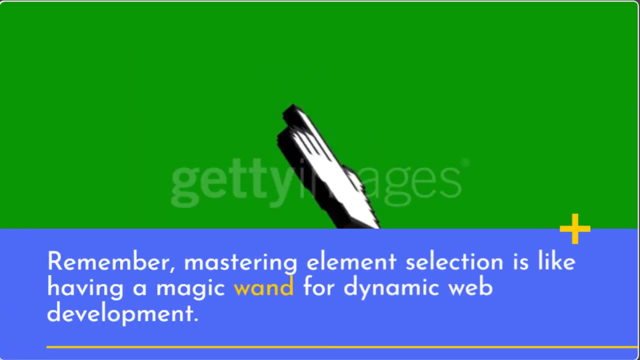 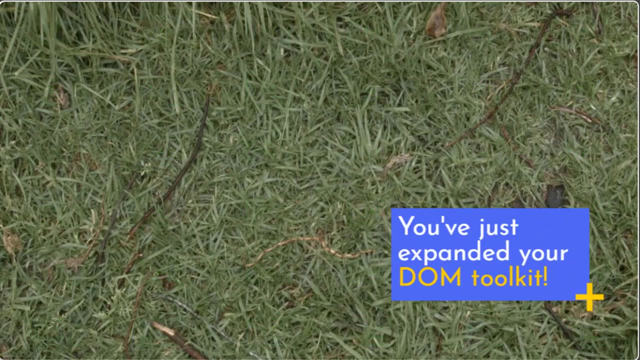 Using the selected elements: consolelog, allListItems, allListItems. And there you have it: various methods to select DOM elements. Remember, mastering element selection is like having a magic wand for dynamic web development. You've just expanded your DOM toolkit. 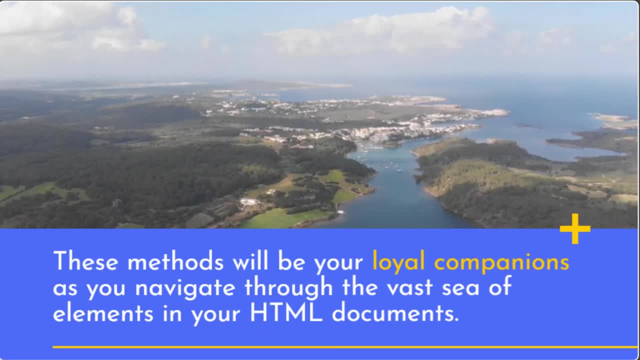 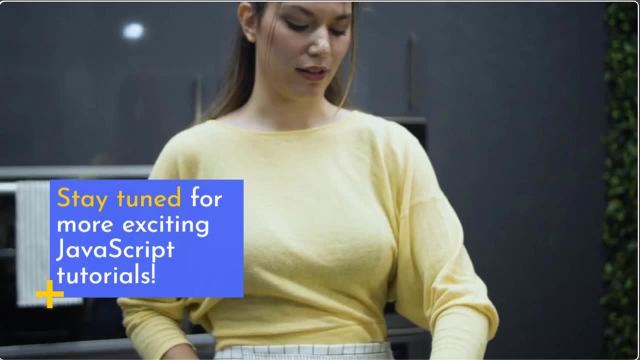 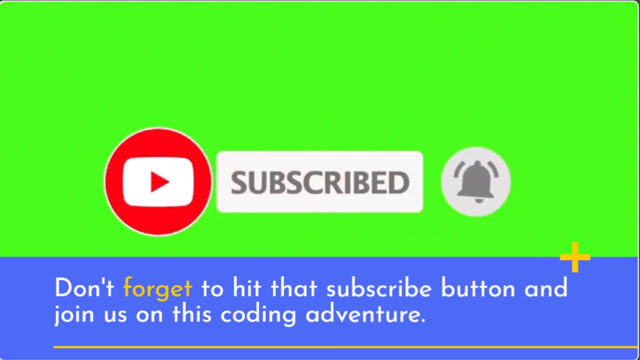 These methods will be your loyal customers. Thanks for watching. Please follow Companions and Companions as you navigate through the vast free of elements in your HTML documents. Stay tuned for more exciting JavaScript tutorials. Don't forget to hit that subscribe button and join us on this coding adventure. 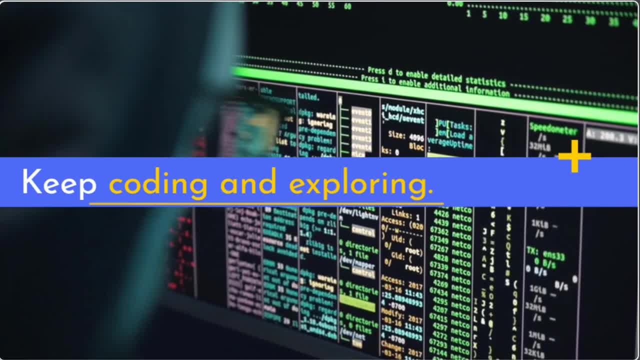 Thanks for tuning in. Keep coding and exploring Until next time. Happy Element Selecting.